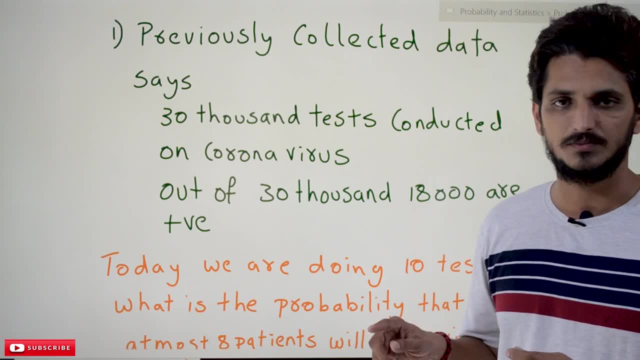 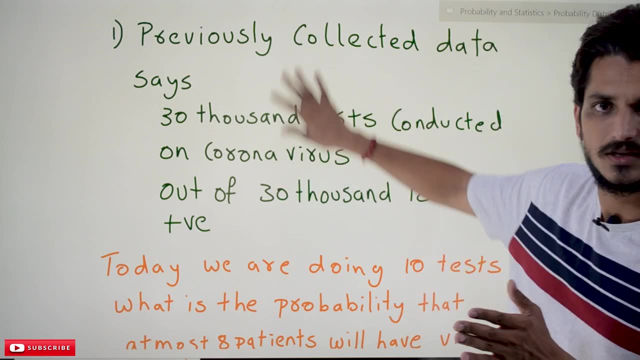 18,000 by 30,000, we will get 0.6.. Means a 60% chance of getting a coronavirus to a person. That is what this data says, So P-value has been provided. From this data we can see that out of 30,000, 18,000 are having positive. means 18,000. 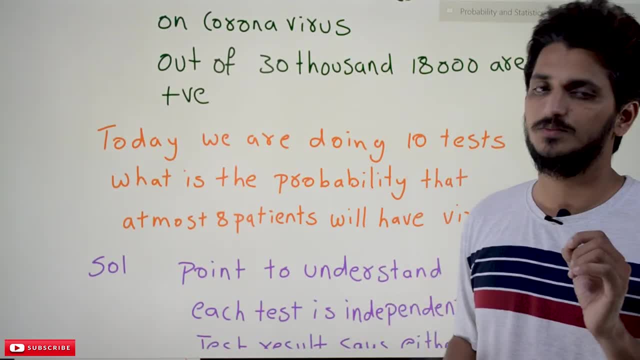 by 30,000.. We will get 0.6.. Means, 60% chance of getting a coronavirus to a person. That is what this data says. So P-value has been provided. Today we are going to speak about we are doing 10 tests. n value has been provided. n is 10 value and what is the probability that? 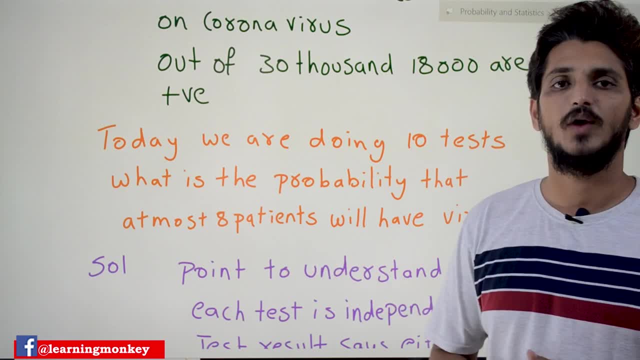 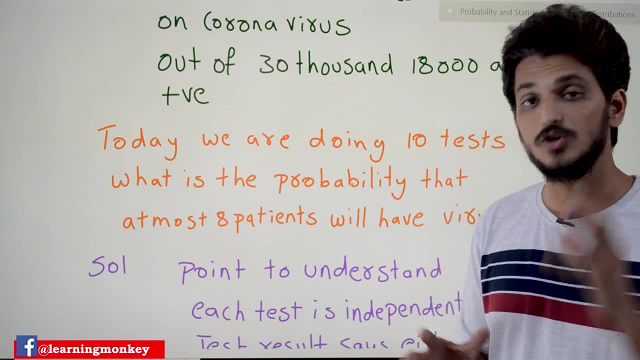 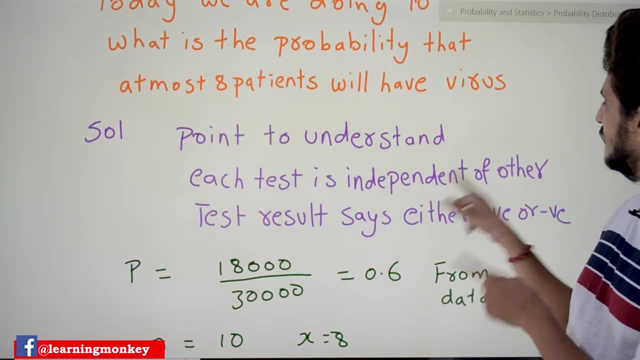 at most 8 patients. x value has been provided. if x value, n value and p value provided, we can apply this to binomial distribution. not only that, you have to check the remaining conditions also. see the point to understand. each test is independent of each other. these are the 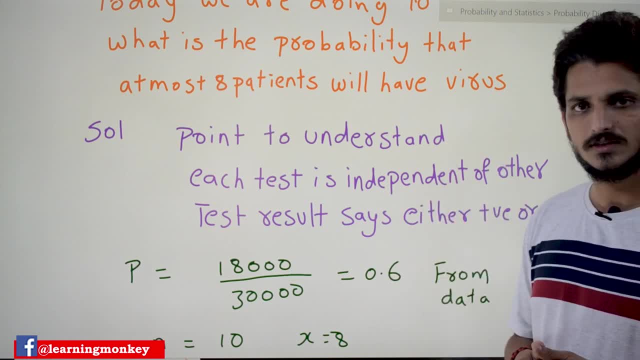 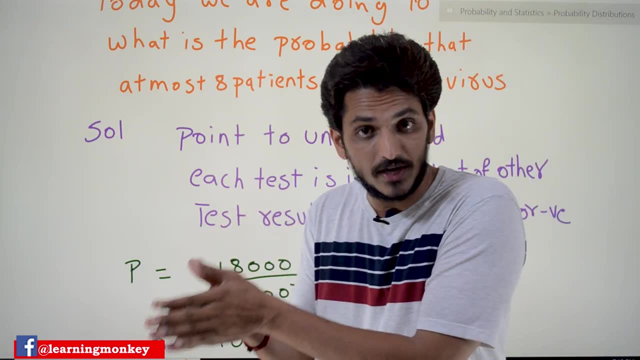 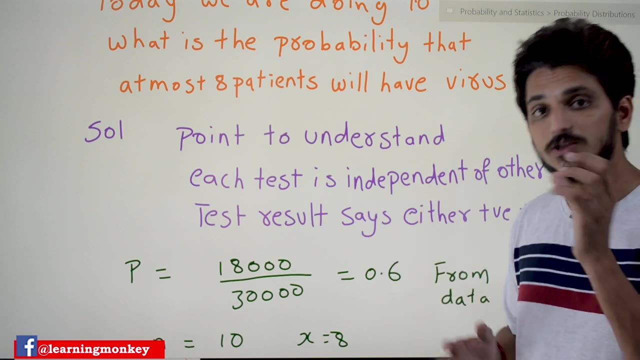 conditions we discussed in our last class. yes, testing you is independent of testing me, so each test is an independent of other test. that is the point you have to understand. that is what binomial distribution says. each, each experiment should be independent of other. yes, here it is. 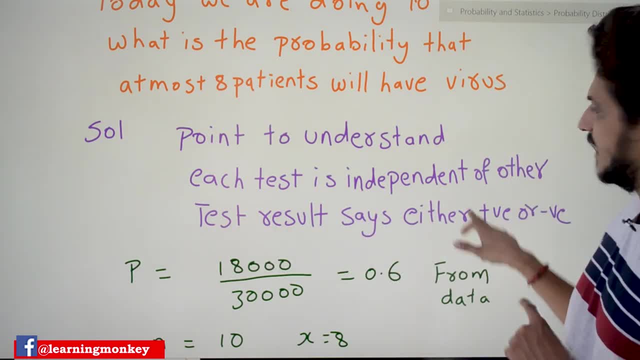 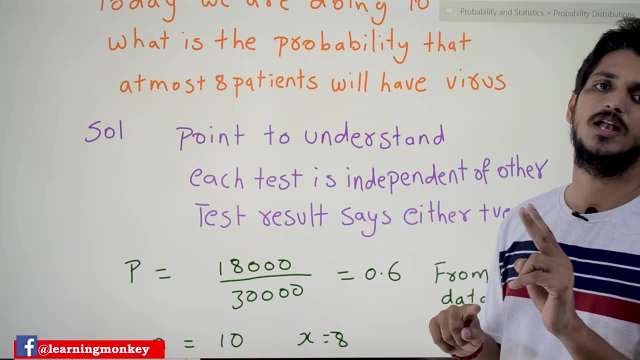 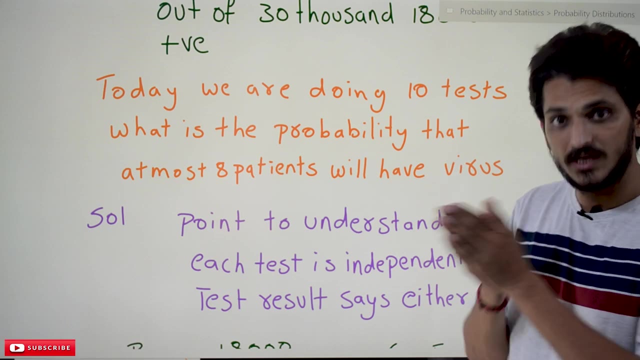 independent of other. next point is: test result. says either positive or negative. means only two values. it is a Bernoulli test: success or failure. now we have made 10 different tests. means if Bernoulli experiment is repeated n times we can apply binomial distribution. that is what we have discussed in our previous class. 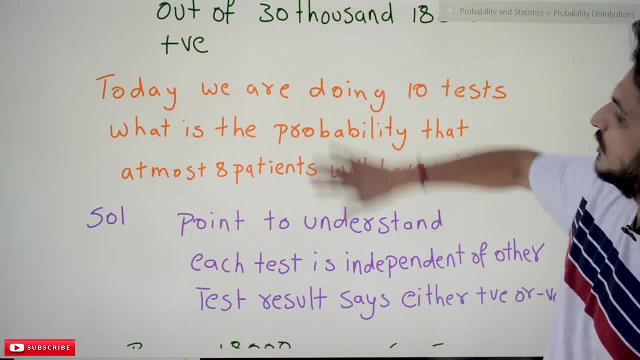 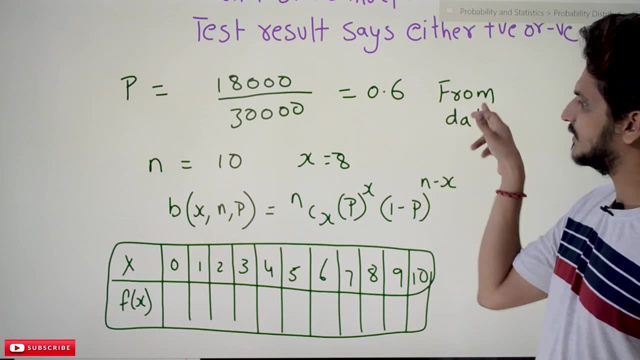 so we can convert this example into binomial distribution. so the p-value is 18,000. by 30,000 that is 0.6. this is given from the data. n is equal to 10. we are going to take n tests out of that how. 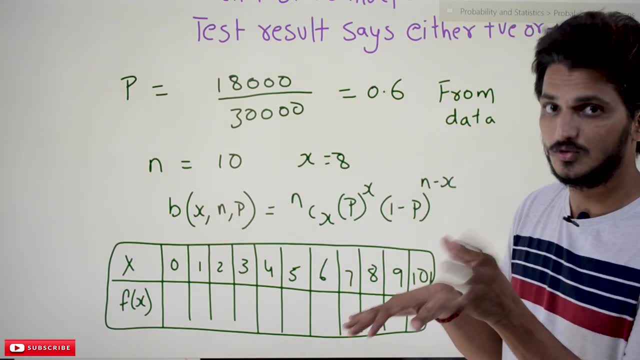 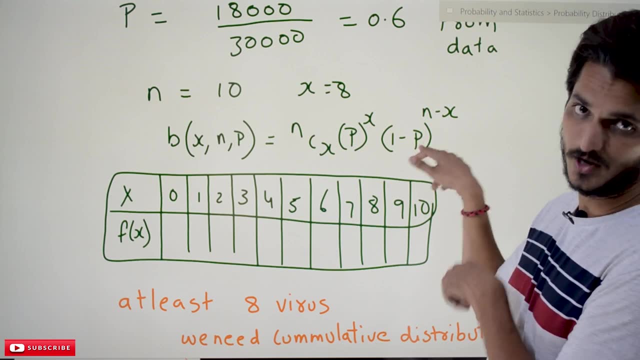 many. x value is 8, at least 8, don't forget that. at least 8. our binomial equation is a: ncx probability is 0.6. 1 minus p means 0.4 power of n minus x. so this is our distribution if you do 10 tests. 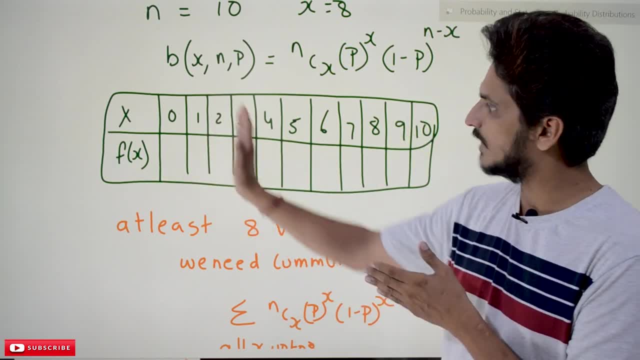 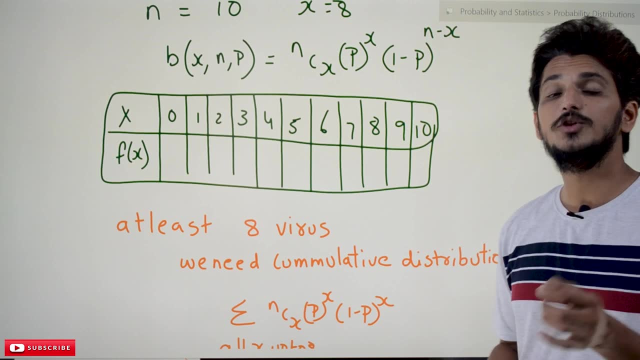 you can have 0, 0 persons having coronavirus, 1 person having coronavirus, 2, so on up to 8. we have to do the cumulative sum, cumulative distribution function. that's why, in real life, cumulative distribution function is 0.6. so we have to do the cumulative distribution function. 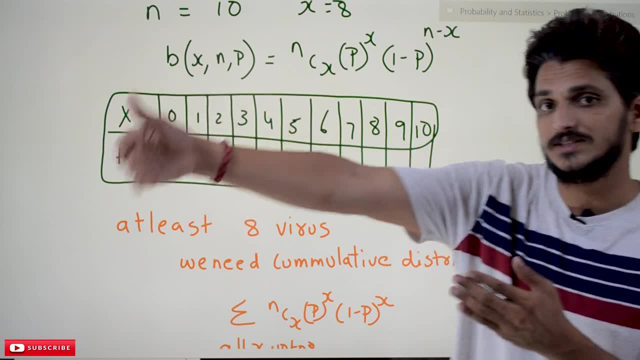 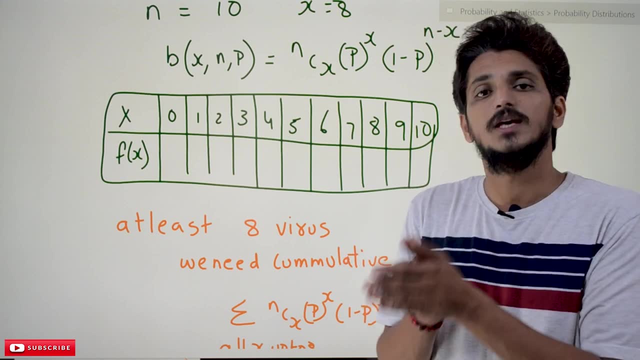 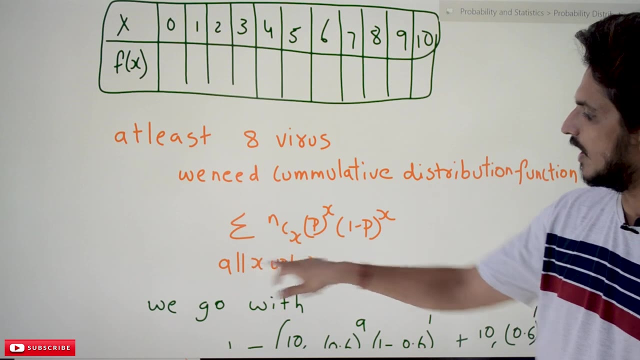 is very, very important. you know previous first examples when we discussed about probability distribution. so we explained what's cumulative distribution function for a given discrete probability distribution. so we have to do that cumulative. we need cumulative distribution function. Sigma all X up to 8. up to 8 we have to summation of all the probability values. this is 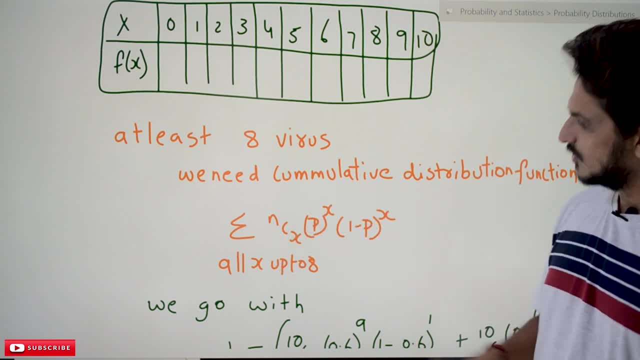 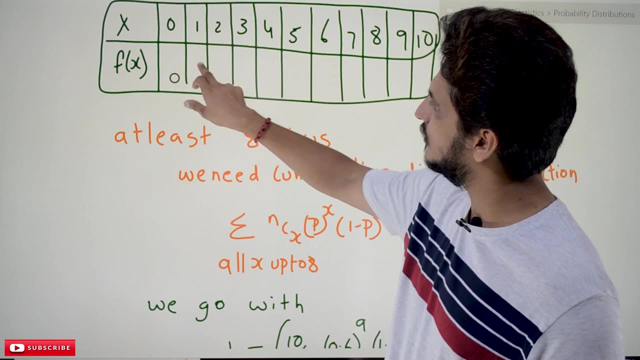 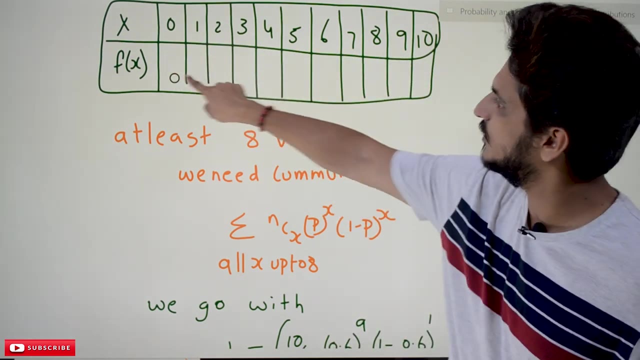 probability mass function for a binomial distribution. so adding all up to 8 is difficult to do the calculation. We have to find NC0,, we have to find NC1, 2, so on up to NC8. summation of all those. Instead of that, adding all these probabilities, here we need to write the probability. 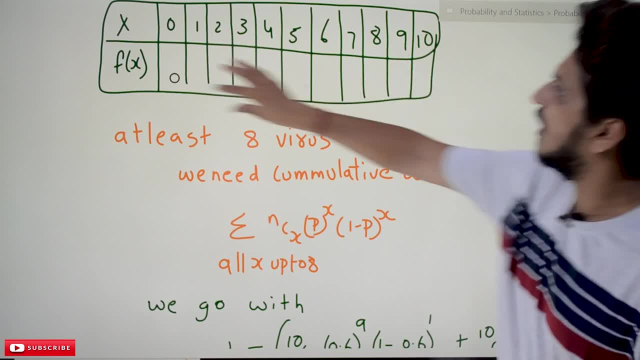 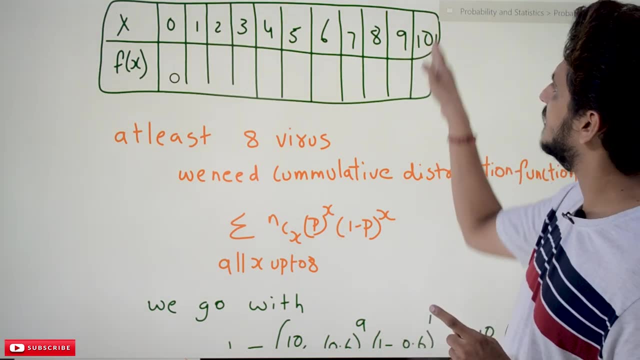 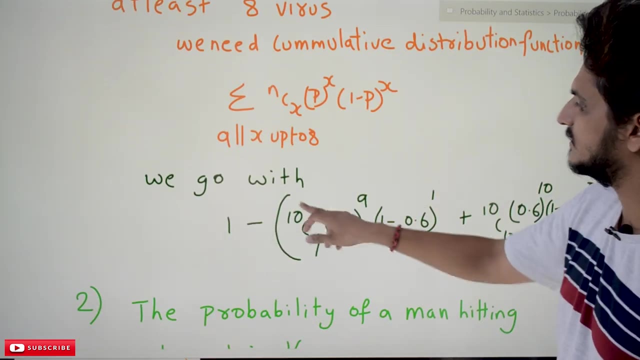 values. Instead of that, adding all the probabilities values, we will get 1.. Sum of all the probability values is 1.. 1 minus NC9- NC10. that gives the same value. We are going with the other way: 1 minus. we go with 1 minus 10C9- 0.6 power- 9,. 1 minus 0.6 power. 1 plus 10C10- 0.6 power- 10 multiplied by 1. 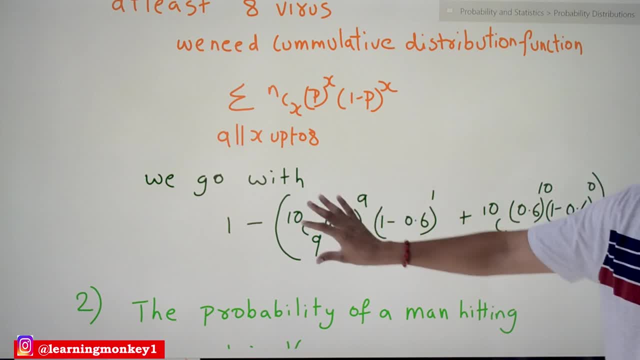 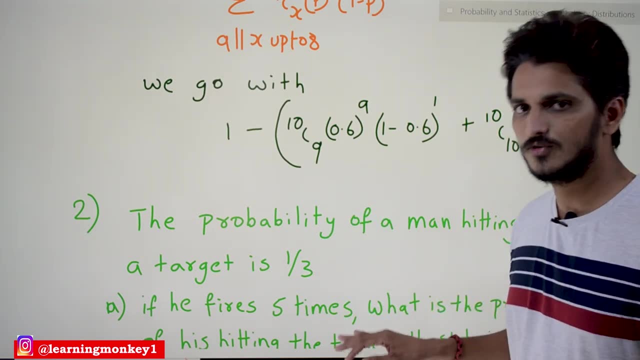 minus 0.6 means 0.4 power 0.. If you calculate this, this is what the probability value you will get. You do the calculation. we are not doing the calculation here, So you try it on your own for better practice. Coming to the second question, so based on this, you have understand. 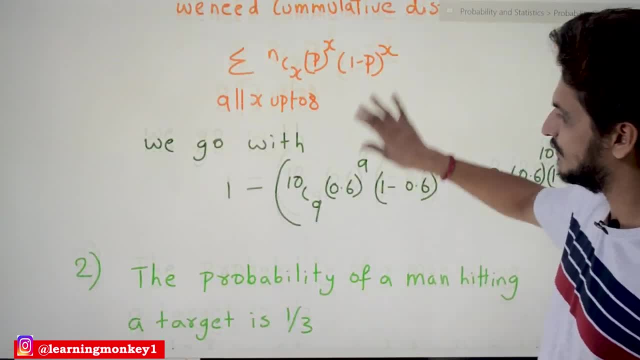 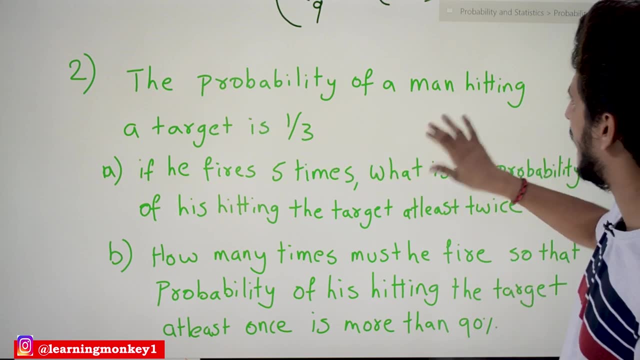 this example. We will go little bit fast for the second example because the concept is the same. So we will go little bit fast for the second example because the concept is well known, So it is very- that is why we are going fast. The probability of a man hitting 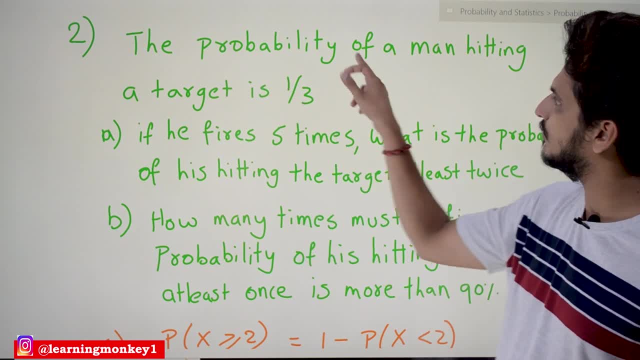 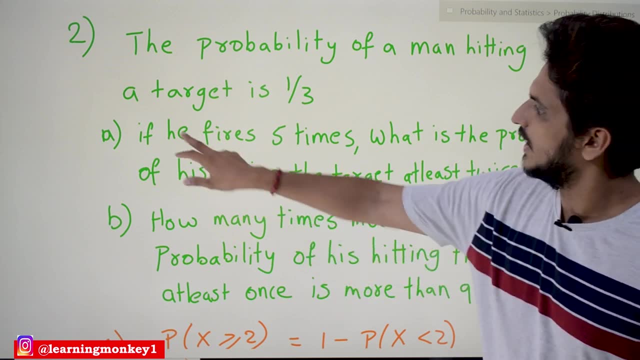 a target is 1 by 3.. It was given that target. the probability of a man hitting the target is 1 by 3.. First question is very easy you have to concentrate much on. second question: If he fires 5 times probability value is given, What is the probability of hitting? 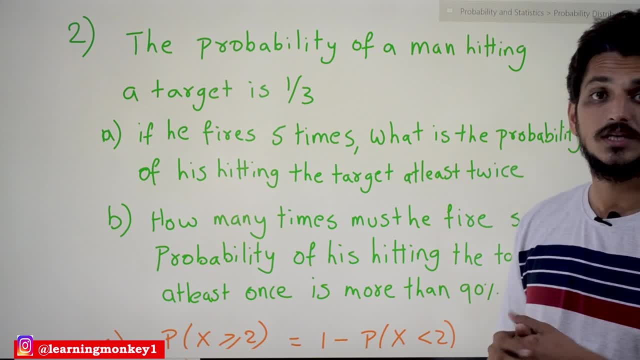 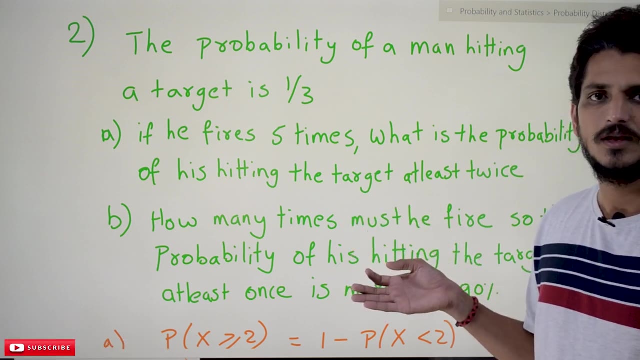 the target at least twice. These are independent events. Yes, Shooting one time is independent of shooting second time, And it is Bernoulli experiment. He may hit or he may miss. We can apply binomial distribution for the first question. Second, 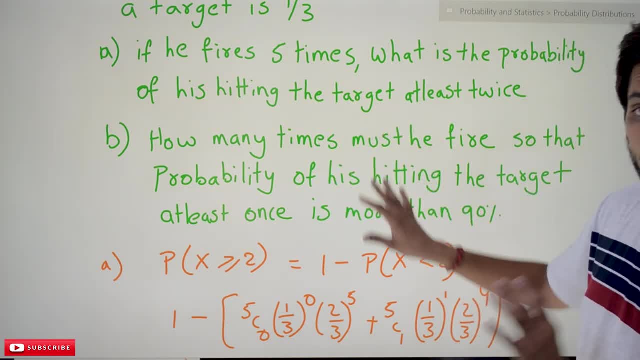 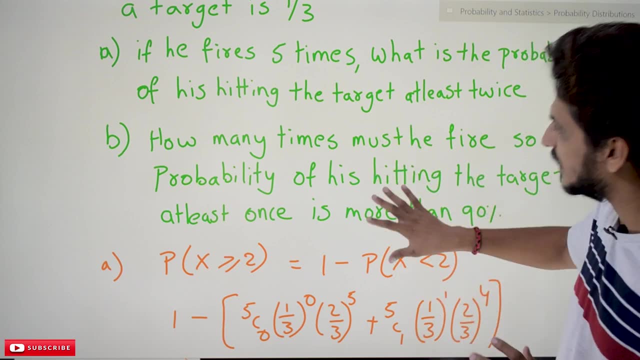 question also: how many times? So this is the question. you have to concentrate much. Think about this question as much times as you want, because most of the times we will apply this in our real life, Not only in this example. You try to concentrate as much as. 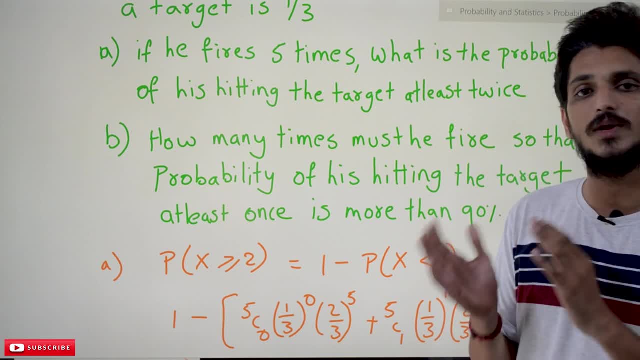 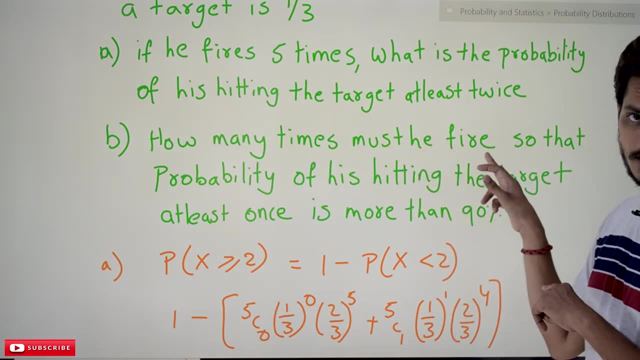 you want You try to elaborate where we can apply binomial distribution in our real life examples. This question is very much used. How many times must he fire? So how many times must he fire so that probability of his hitting the target at least once is more than 90%? 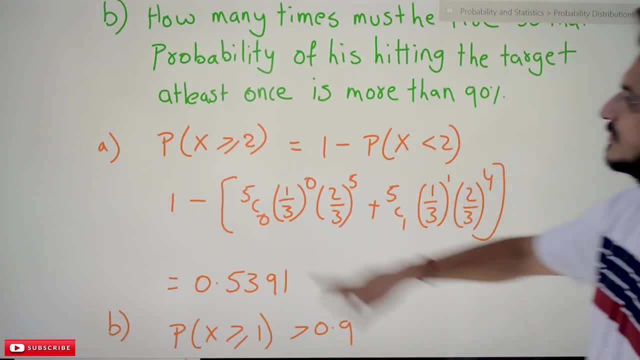 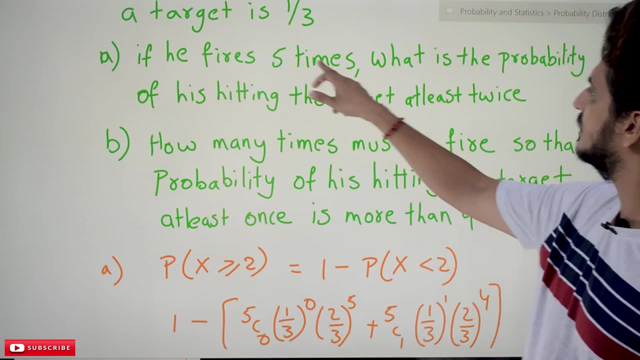 So this is very important to understand. So coming to the first question: probability of X greater than or equal to 2.. This is the question they have asked. X greater than or equal to 2 means here probability value is given 1 by 3.. N value is given He. 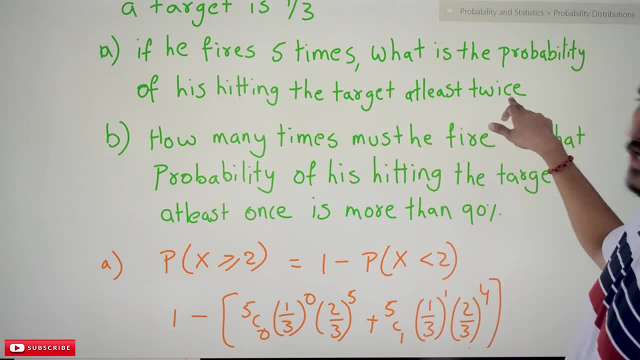 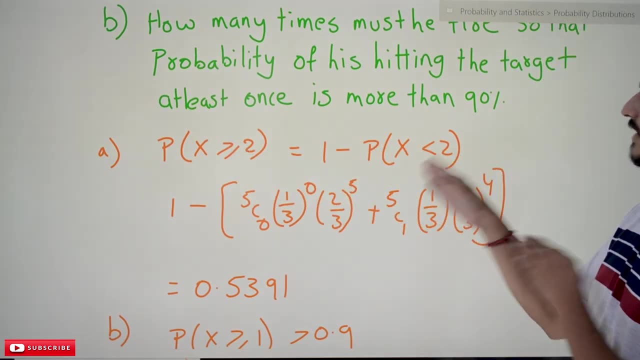 is shooting 5 times. What is? the X value is given Twice, So probability of X greater than or equal to 2.. Instead of finding this, we can go with 1 minus probability of X less than 2.. Summation of all the probabilities is equal to 1.. That is why we are going with 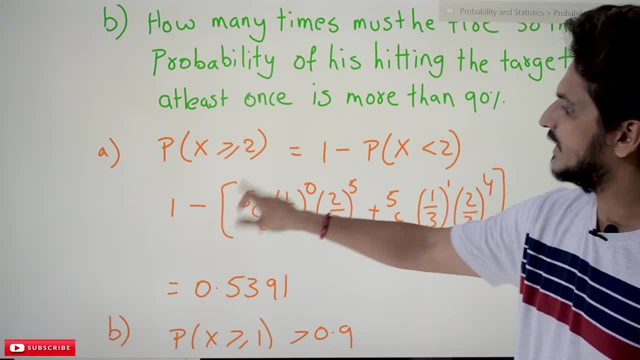 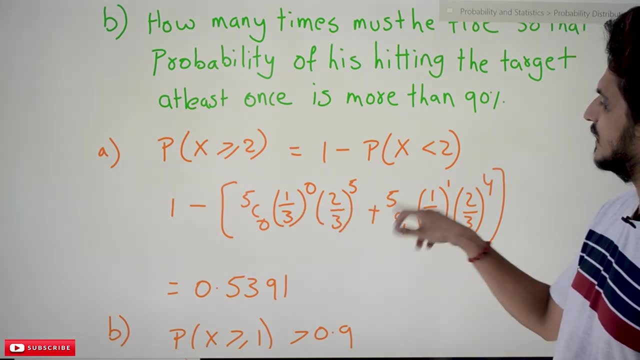 other way. It is easy for the calculation: 1 minus 5C0, 1 by 3 power 0, 2 by 3 is the miss probability. This is hit probability Power 5 plus 5C1, 1 by 3 power 1, 2 by 3 power 4.. If you find this, the final value is 0.5391. 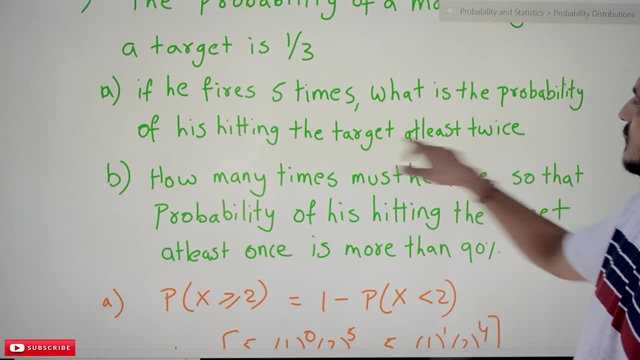 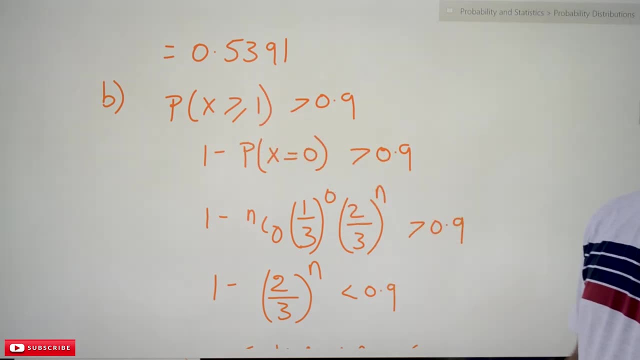 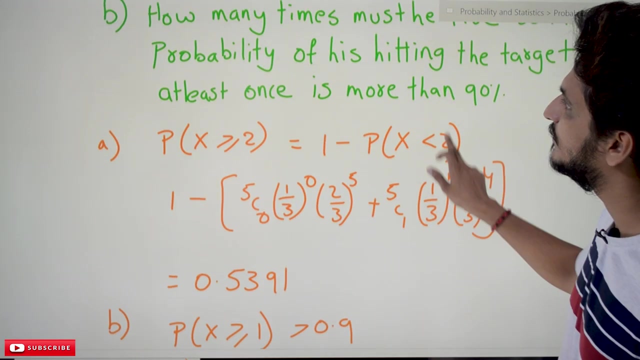 This is the probability he is going to hit for the first question, At least twice. Coming to the second question, probability of X greater than or equal to 1 is greater than 0.9.. From the question it was given that how many times? how many times must he fire? 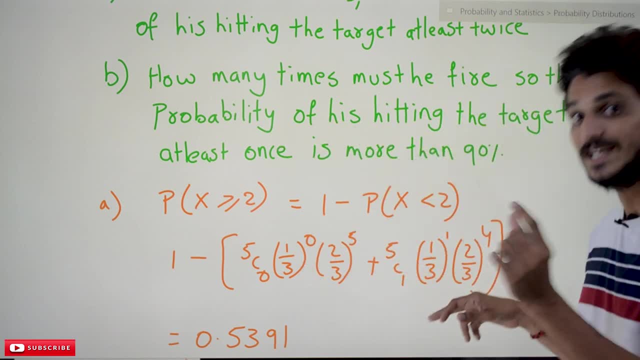 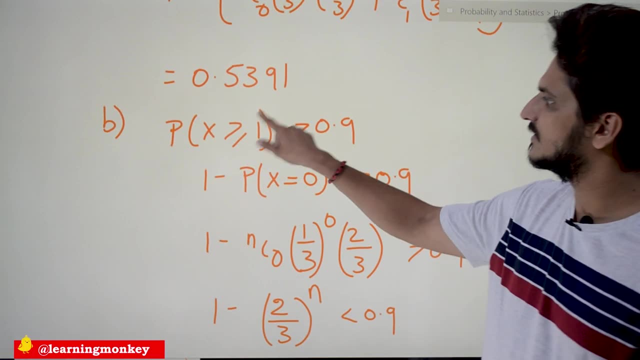 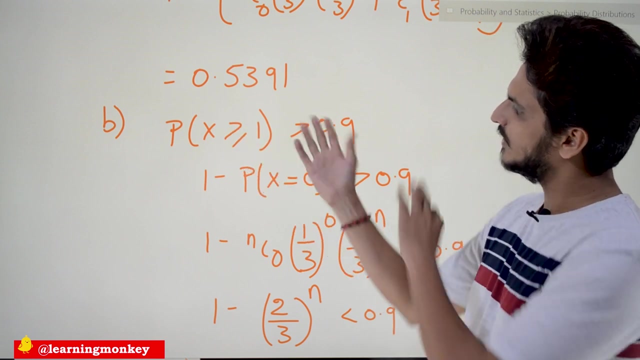 so that probability of his hitting the target at least once is more than 90%. So that's why probability of X greater than or equal to 1 greater than 0.9.. From this, if you want to find the probability of X greater than or equal to 1, we can convert this into 1. 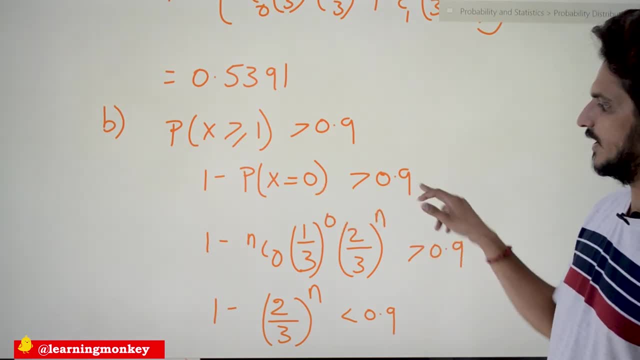 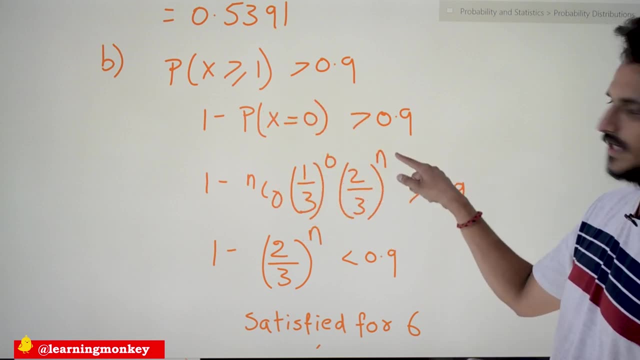 minus, probability of X is equal to 0, greater than 0.9.. 1 minus. if you find this, probability of X is equal to 0,. NC0, 1 by 3 power 0, 2 by 3 power n. We need to find.